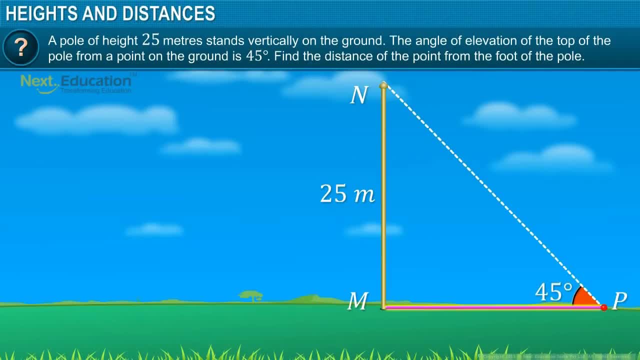 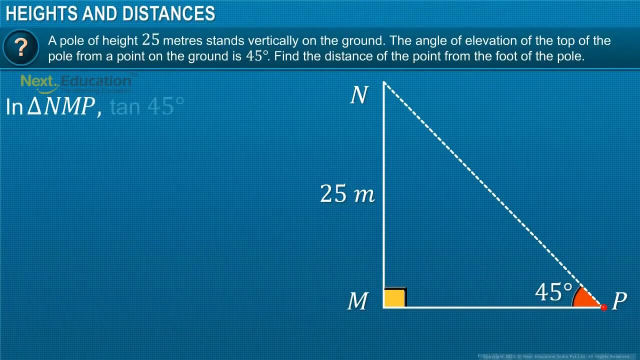 We need to find the distance of the point P from the foot of the pole M. Here, triangle Nmp is a right angled triangle. In the triangle, tan 45 degrees is equal to tan 45 degrees is equal to tan 45 degrees. N divided by: 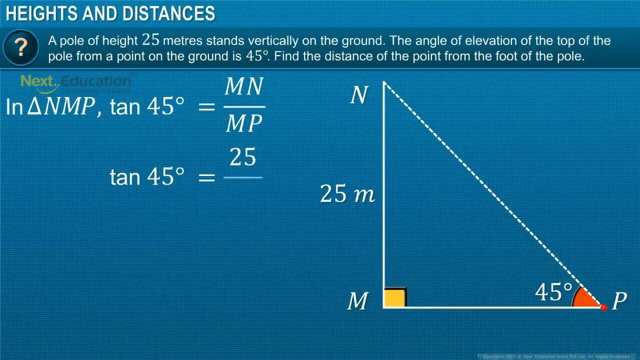 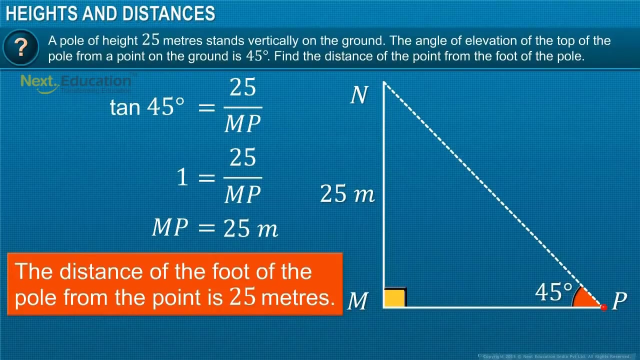 Let's substitute the value of Mn. Mn is equal to 25 meters. The value of tan- 45 degrees- is equal to Rearranging. we get the value of mp, that is, the distance of the foot of the pole from the point. 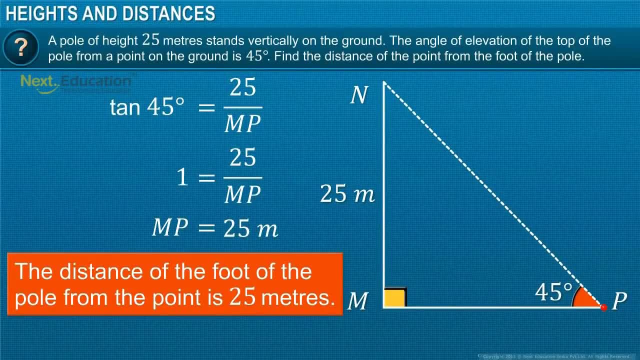 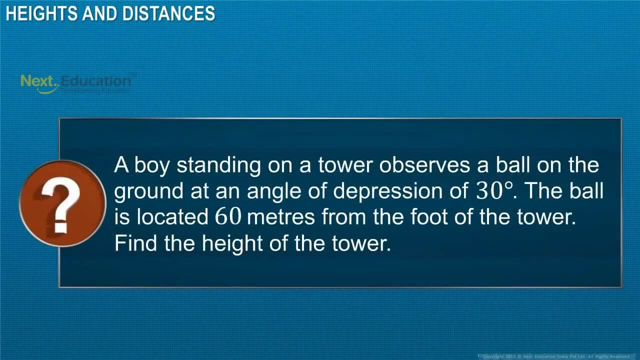 is equal to 25 meters. Let's look at another example. A boy standing on a tower observes a ball on the ground at an angle of depression of 30 degrees. The ball is located 60 meters from the foot of the tower. Let's find the height of the tower using the angle of depression. 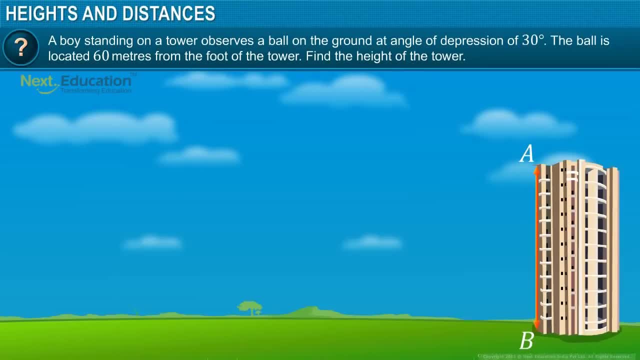 Let a b represent the tower. The ball is located 60 meters away from the foot of the tower. The boy observes the ball at an angle of depression of 30 degrees. When this line is joined, a triangle is formed Here. the side AC makes an angle of 30 degrees with the horizontal AP. 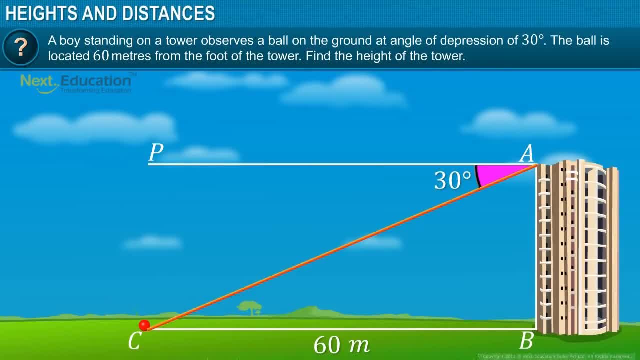 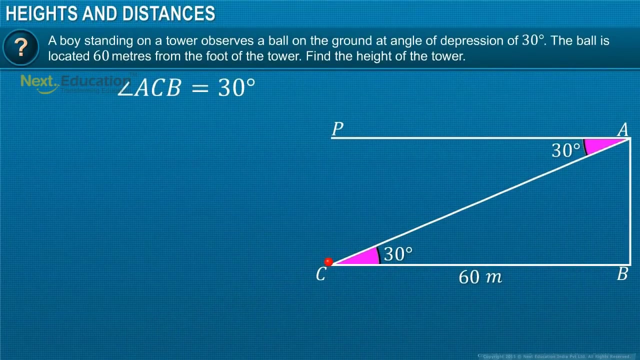 Considering the side AC as the transversal of parallel lines AP and BC, angle ACB and angle PAC form a pair of alternate angles, Hence they are equal. Therefore, angle ACB is equal to 30 degrees In the triangle ABC. 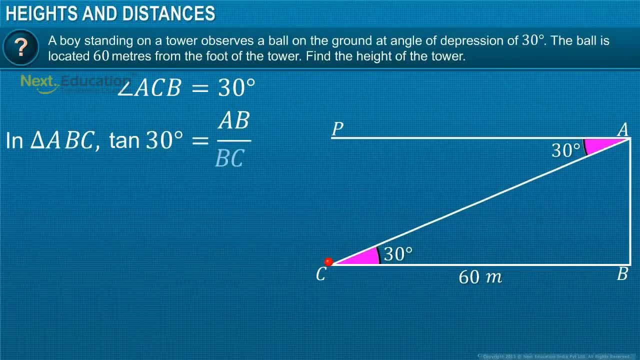 tan 30 degrees is equal to AB divided by BC. Substituting the values, tan 30 is equal to 1 by root 3 and BC equal to 60 meters, We get AB by 60 equal to 1 by square root of 3.. 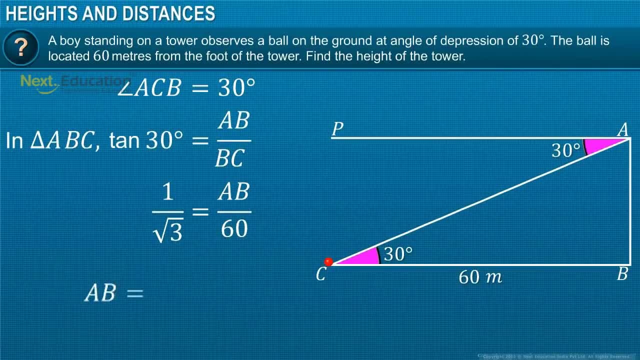 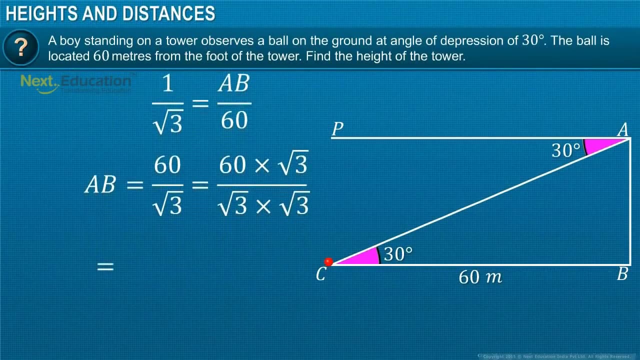 Rearranging the expression, we get AB equal to 60 by square root of 3.. In the triangle, tan 30 is equal to 60 by square root of 3.. In the triangle, tan 30 is equal to 60 by square root of 3.. 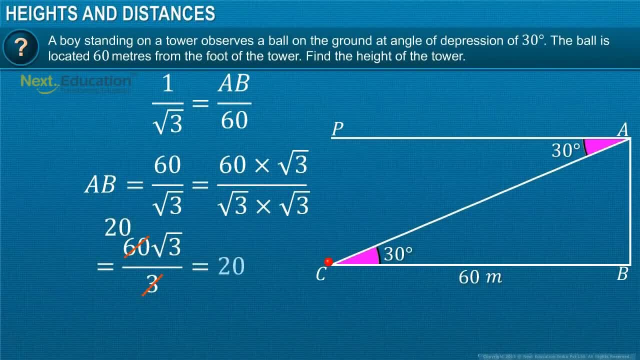 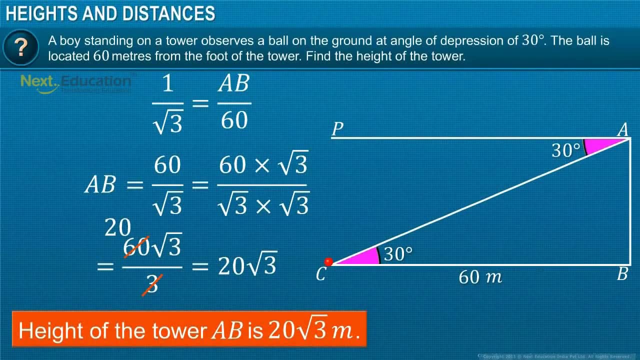 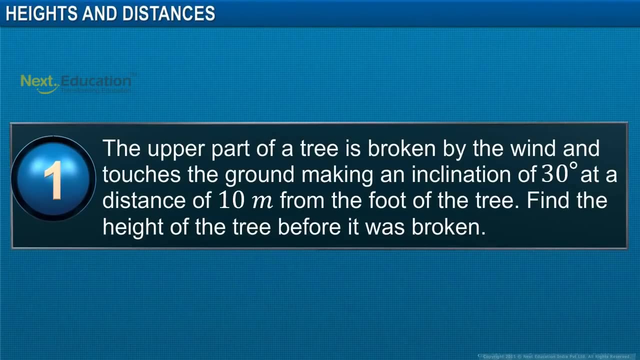 On simplifying, we get 20 multiplied by square root of 3 meters, which is the height of the tower. The upper part of a tree is broken by the wind and touches the ground, making an inclination of 30 degrees at a distance of 10 meters. 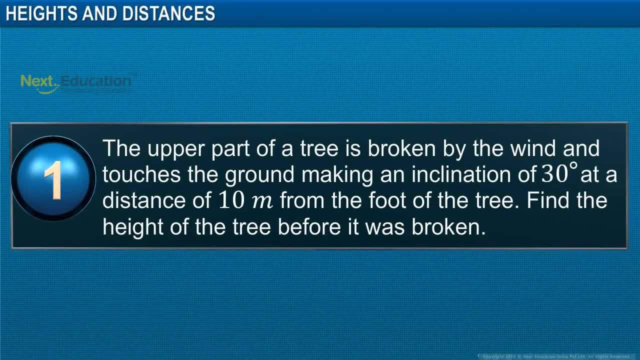 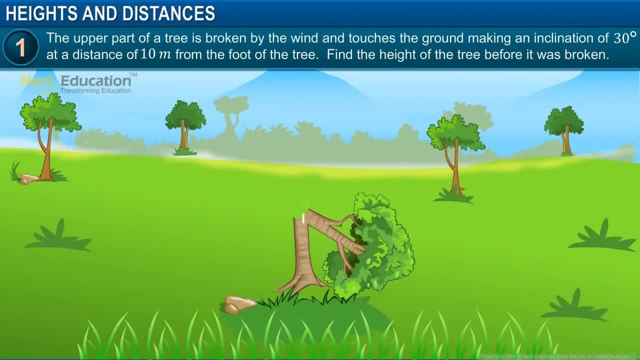 from the foot of the tower foot of the tree, Find the height of the tree before it was broken. From the figure, let the two broken parts of the tree be AB and AC, Given that the angle of inclination from C is 30 degrees and the distance between the foot of the tree and the broken part touching 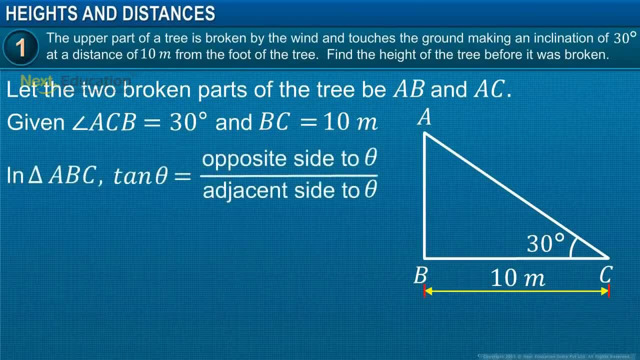 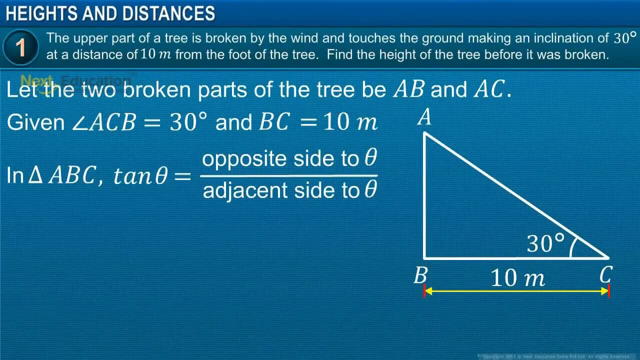 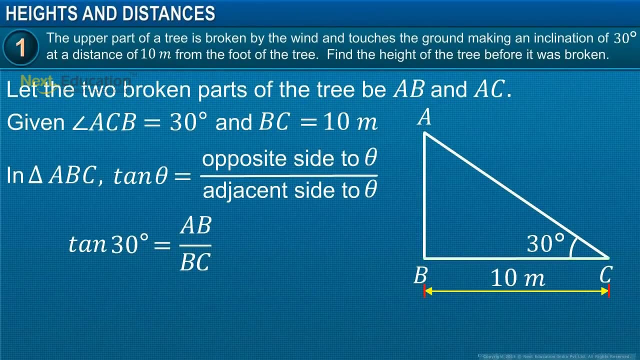 the ground is 10 meters. In triangle ABC tan theta is equal to opposite side to theta. divided by adjacent side to theta, Tan 30 degrees is equal to AB divided by BC. Substituting the values and simplifying, we get AB is equal to 10 upon root, 3 meters. 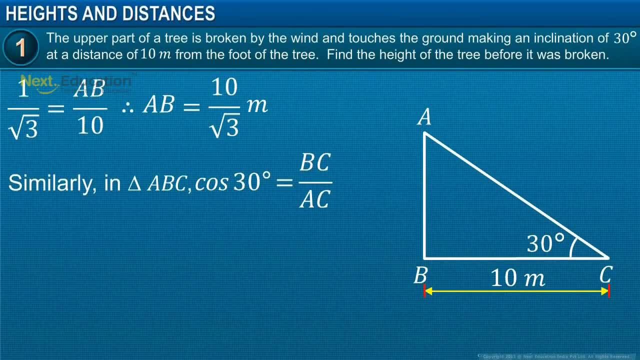 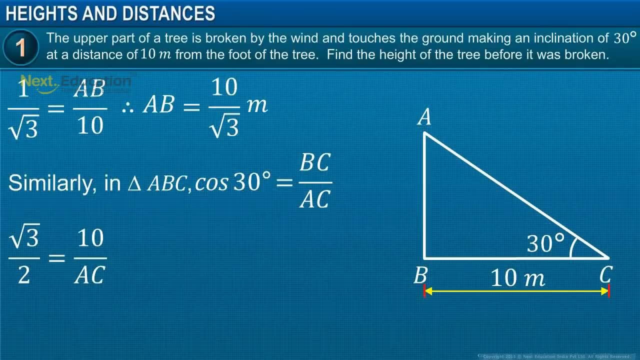 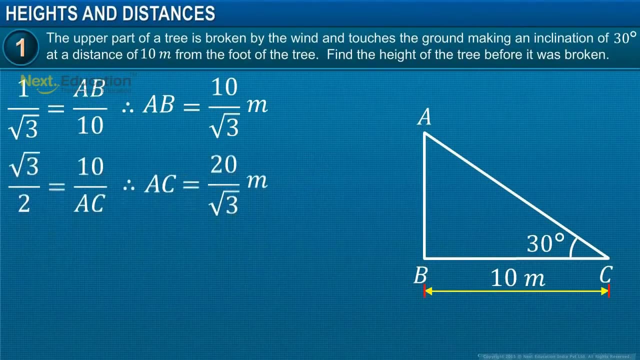 Similarly, in triangle ABC, cos 30 degrees is equal to BC divided by AC. Substituting the values and simplifying, we get AC is equal to 20 upon root 3 meters. Therefore, the height of the tree before it was broken is equal to AB plus AC. Substituting the values of: 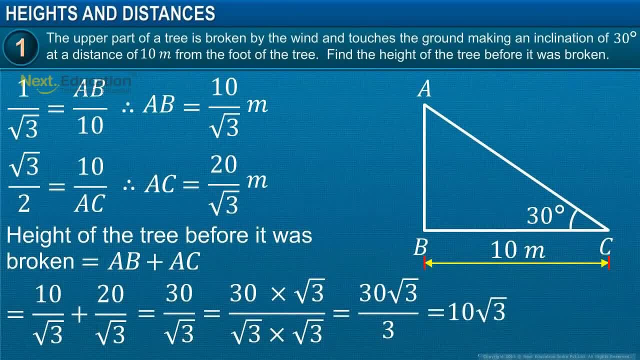 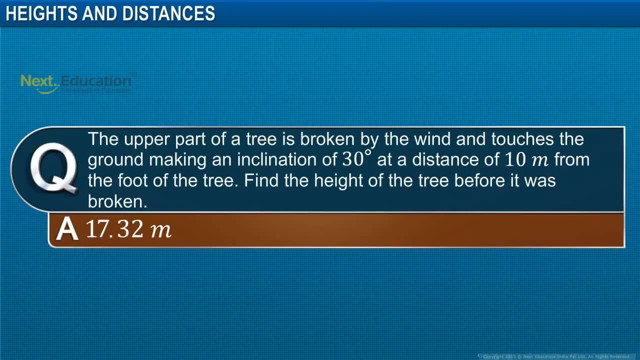 AB and AC. we get the height of the tree. Given the four corners are bent, the two sides of the tree are Zeiten. This is equal to H, who is the two corners of the tree. Similarly, we can open the edges of both sides of the tree and remove either the corner. 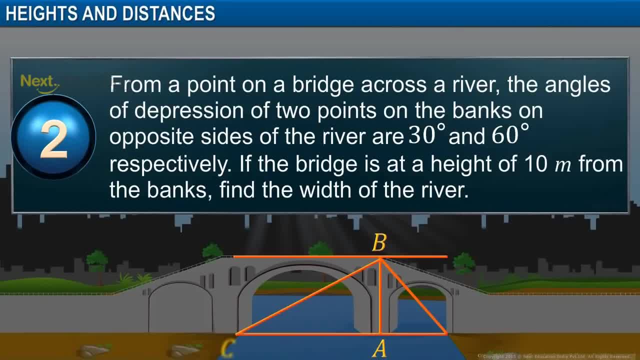 half away, or the corner half away, with the same angle and the third side of the twoien cups. We will1 Now for the right angle and the box in the number of sides facing the left and right angles are same 넘. 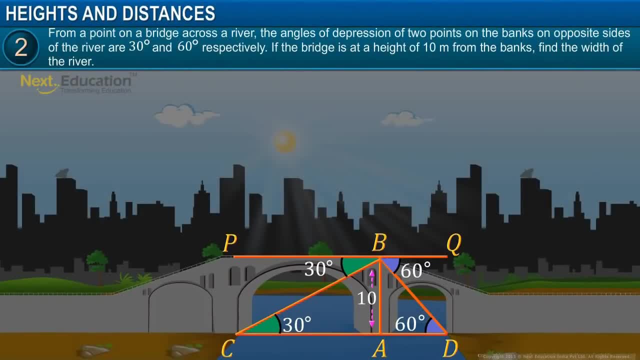 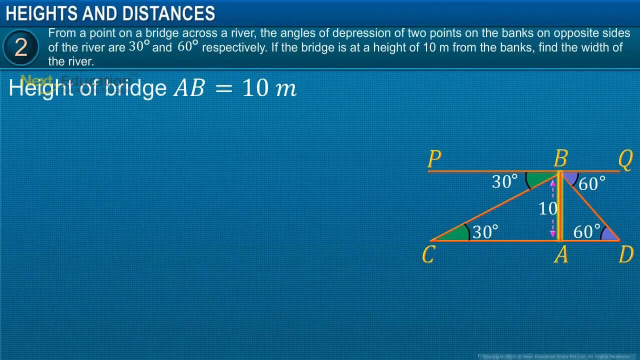 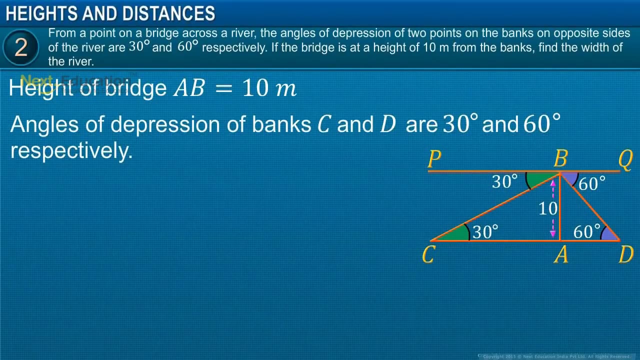 B, The height of the bridge is 10 meters and the angles of depression of points C and D on the banks are 30 degrees and 60 degrees respectively. In the figure, let us assume AC is equal to X and AD is equal to Y. 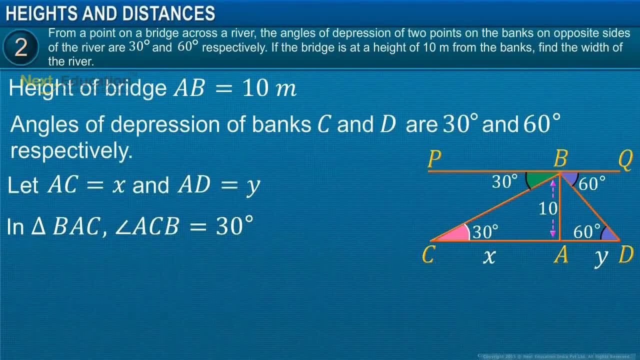 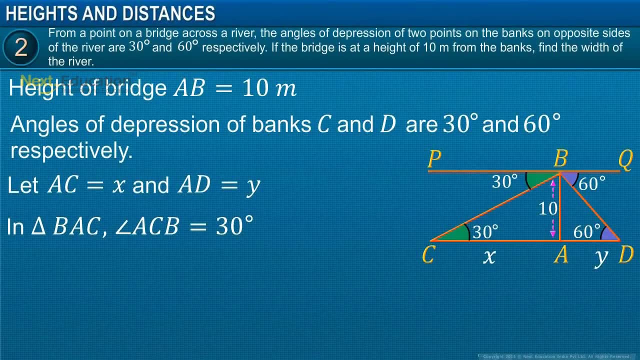 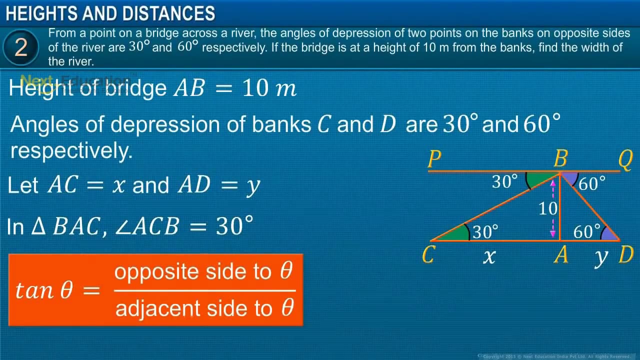 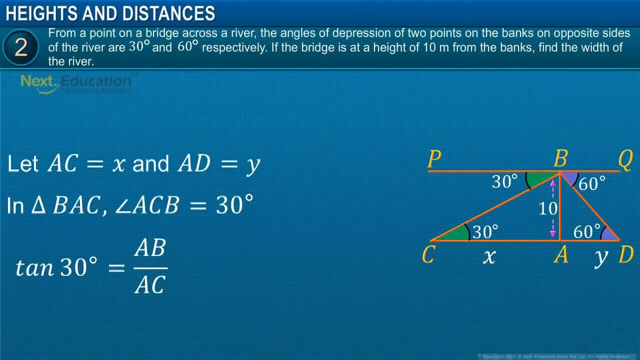 In triangle BAC, we know that angle ACB is equal to 30 degrees. since angle ACB and angle CBP are alternate angles, We know that tan theta is equal to the opposite side to theta divided by the adjacent side to theta, which can be written as: tan 30 degrees is equal to AB divided by AC. 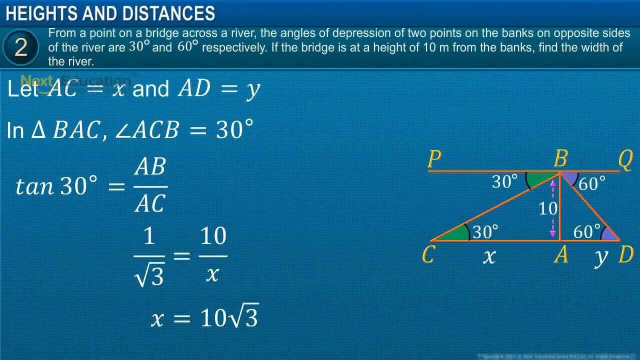 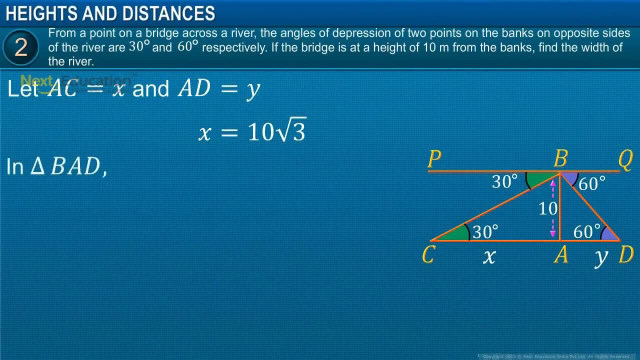 On substituting the values of tan, 30 degrees, AB, AC and simplifying, we get the value of X as 10 root 3.. Similarly, in triangle BAD angle, ADB is equal to 60 degrees. Substituting the values of tan, 60 degrees as root 3 and AB as 10, and simplifying we 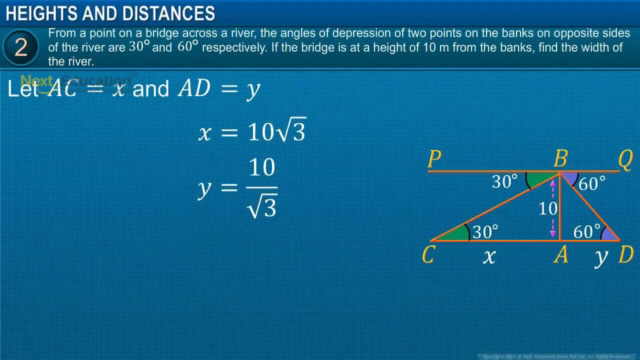 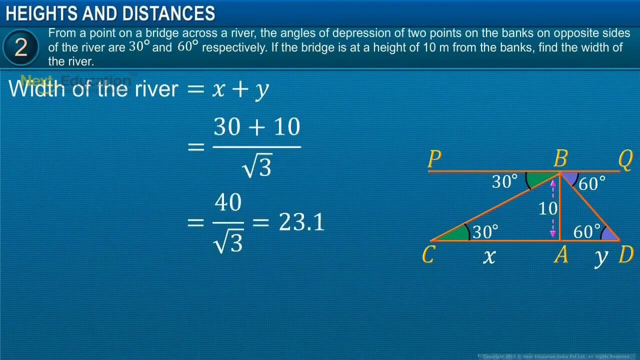 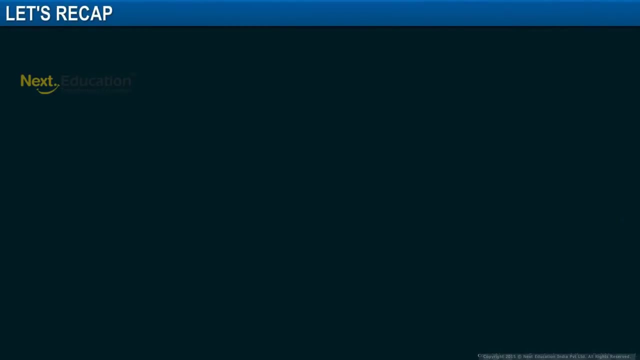 get. the value of Y is equal to 10 upon root 3.. From the figure, the width of the river is X plus Y. On substituting the values of X and Y and simplifying, we get the width of the river as 23.1 meters. 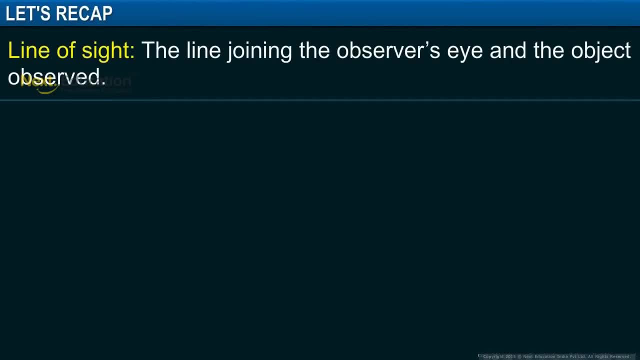 In this module you learnt that the line joining the observer's eye and the object observed is called line of sight. The angle between the horizontal axis and the horizontal axis is called line of sight. The angle between the horizontal axis and the horizontal axis is called line of sight.